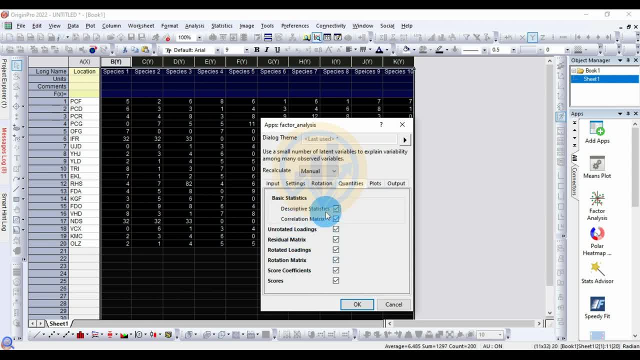 The quantitative select for the all, the checkbox, The descriptive statistics correlation matrix and unrotated loading, the residual matrix, The all the score values, the check, the tick box, Then next one for the plat, The plat, The scar plat, Variation plat, also the tick. 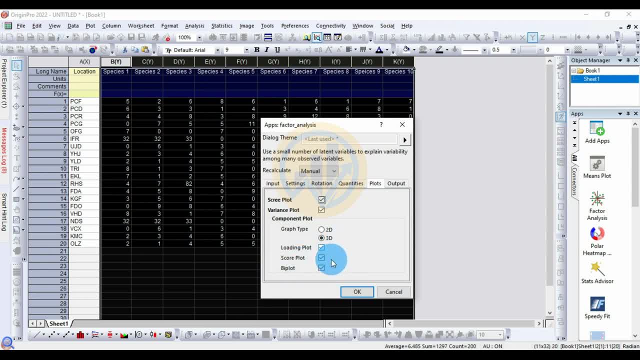 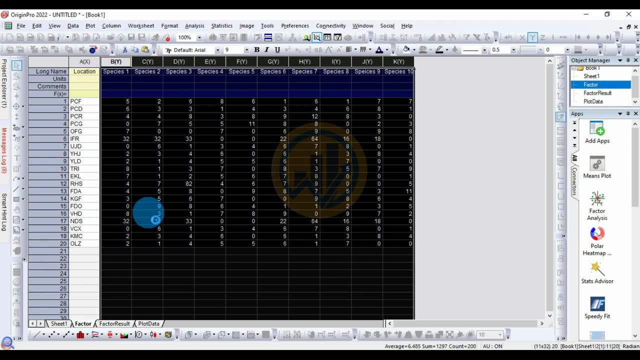 user would be not good in PCS case. Next one for the philosophy of student knowledge in popularity, biplaton. so the check, click the check box. then click the ok button. now get the factor analysis result. okay, open the first one, the basic statistics. click the. 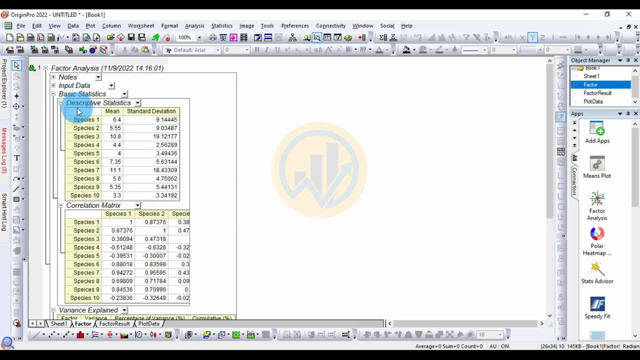 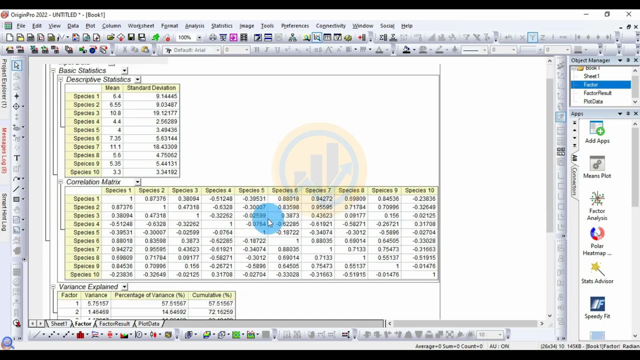 plus icon the basic statistics. for the descriptive statistics, the 10 species mean value and descriptions value, standard deviation value for the present in that descriptive statistics. the next one for the correlation matrix: the correlation matrix for the species to pieces correlation, the species one, the correlation for the positive in the PC 1, 2, 3 and 6, 7, 8 and 9. also the 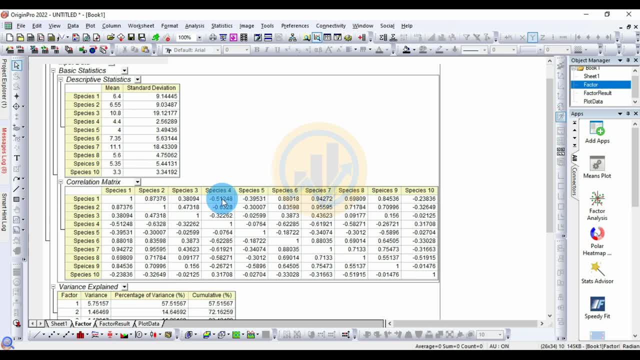 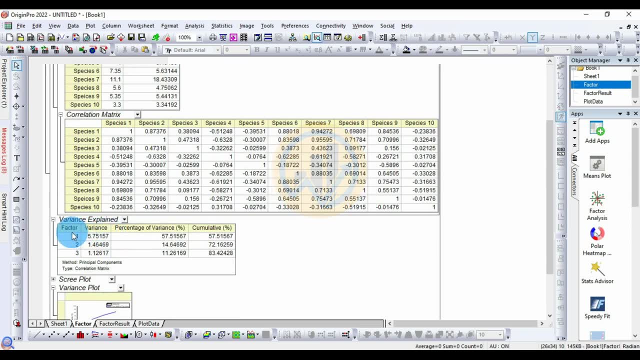 positive correlated the species, one negative correlated for the PC 4 and PC 5 and final for the PC 10. the next one table for the variation explanation. the variation explained for the factor 1 and 2: 3. the variation highest present in the factor 1. 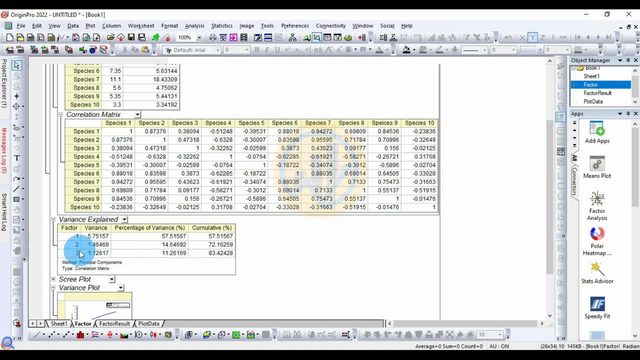 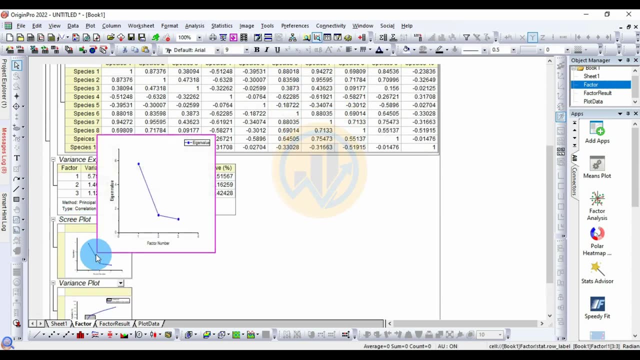 5.75. the percentage of various in the highest presented in the factor one. fifty-seven point fifty one. the next cumulative percentage for the highest present. the cumulative presented for the factor three: 83 point 42. the next one. for the scar Cloud, the click the plus icon, the dump clip or the scar plot open. 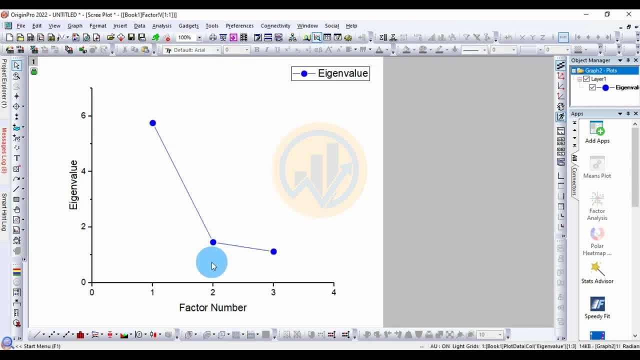 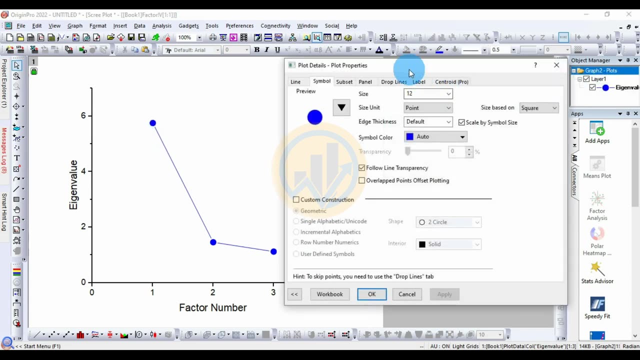 then new window, further scape ladder. this is a factor one under two, three. then I can value the highest percent for the factor one and lowest present value for the factor three. the double click for the icon open the new plot details the change for the symbol. 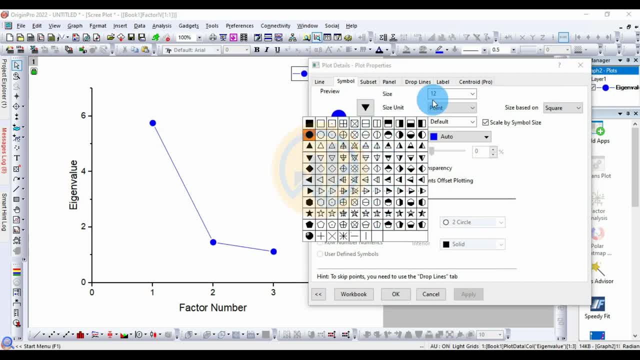 the different symbols available: the choose symbol, different symbol. and the next one for the size, the increased word size or decreased size. the next one for the change color for the symbols, the variation color available in the symbols. the next one for the lines. 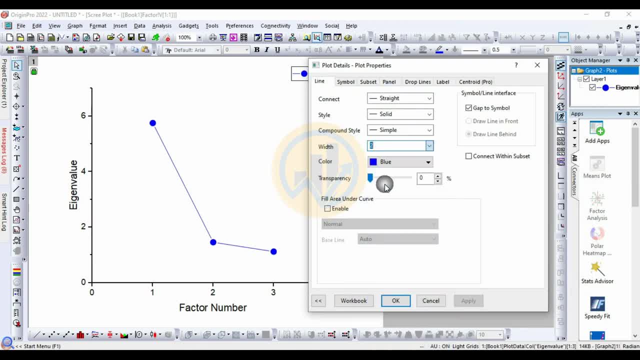 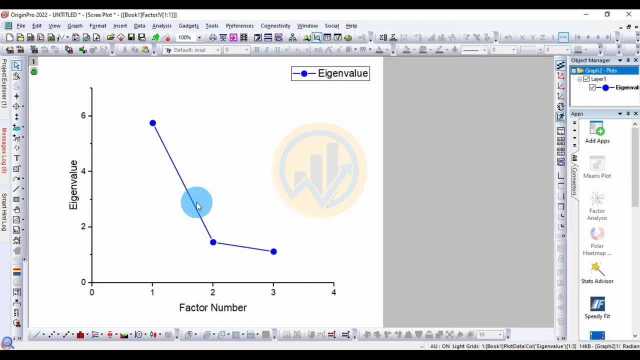 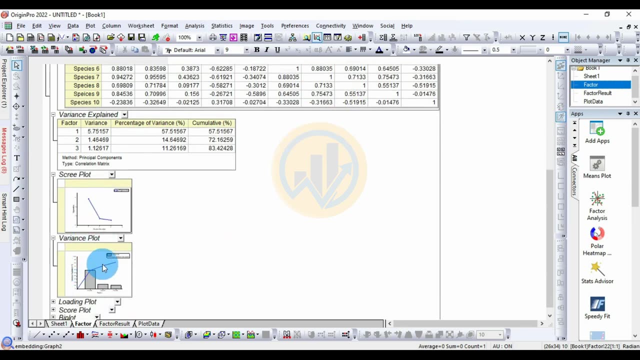 the lines is a change for the width. increase rate, increase the width under the style of the line. the next one for the click. okay, then this is for the square plot, then next one for the variation plot. double click for the variation plot. 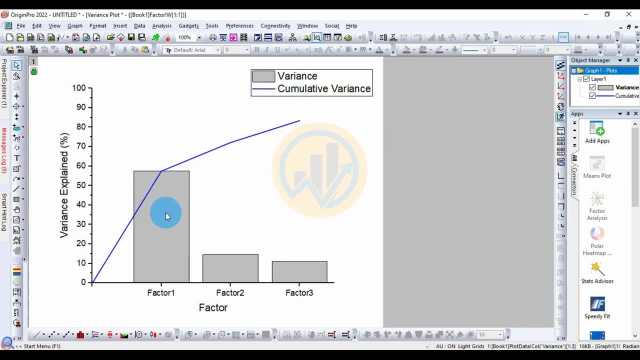 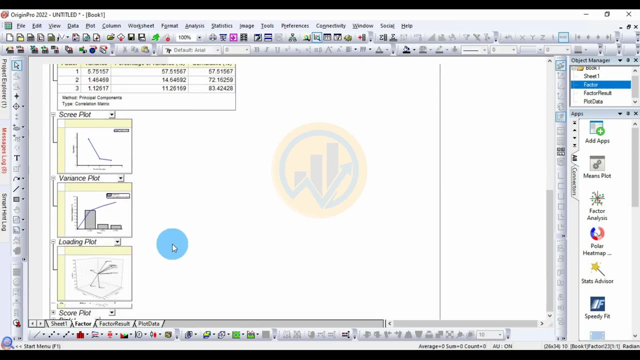 open the new window. then variation value: the highest present in the factor one and lowest for the factor three. this line for the cumulative lines, then variation explained, then next one plot for the loading plot. double click for the loading plot. open the new window for the loading plot. 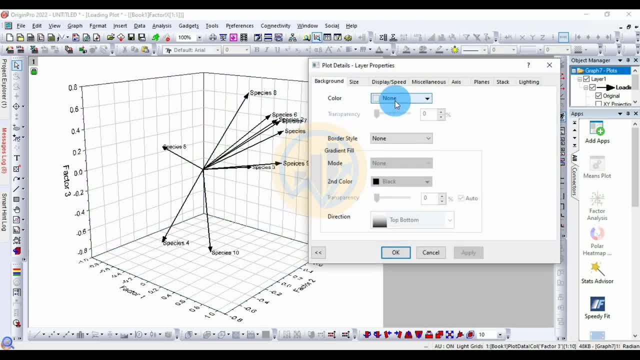 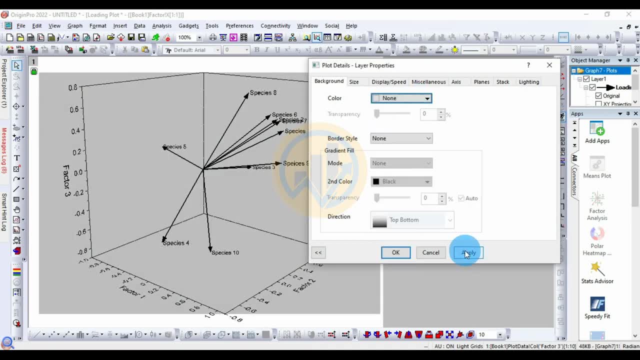 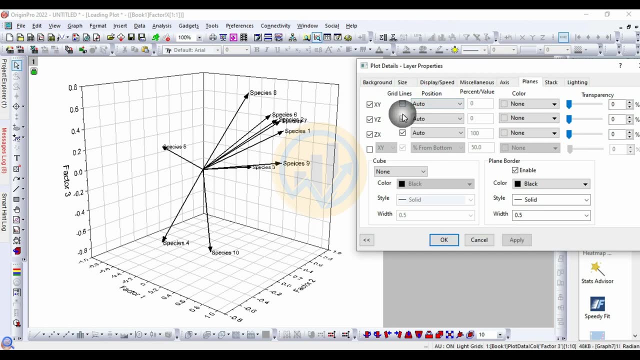 double click for the center center plot. then first one for the background color change. for the background color- now unknown color. the next one for the panels. then remove for the background color change for the this grand line. remove the grand line checkbox. 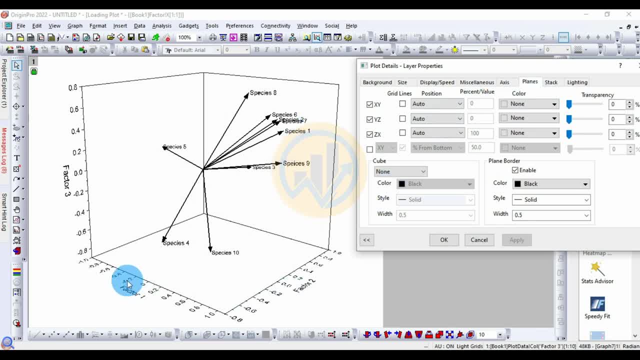 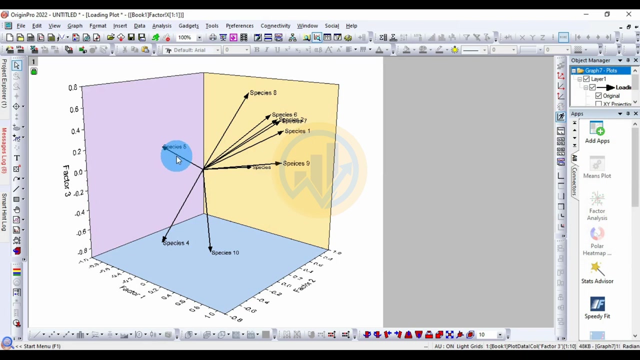 then apply the center grand line change for the factor one, two and three the colors. then factor one color change. second one color, change the third one color. then apply change for the background color. then click the ok button. then single factor percentage in the factor three is for the species five. 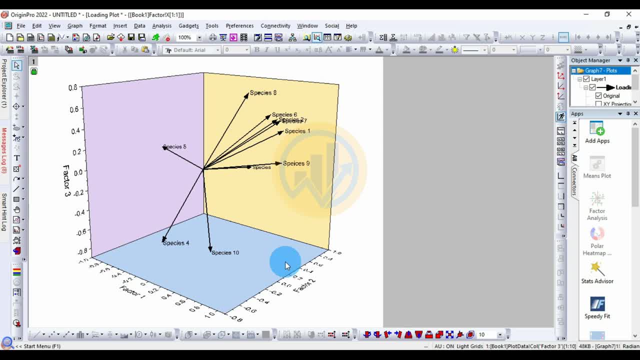 then fixes four and pieces ten present in the factor one, the large of species present in the group for the factor two, the nine one, seven, two, six, eight. also the present in the factor two. this is the loading plot. 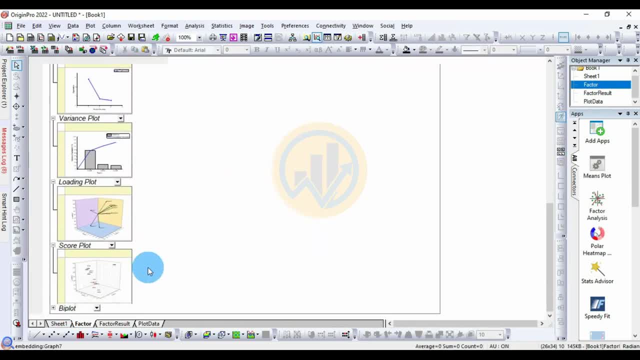 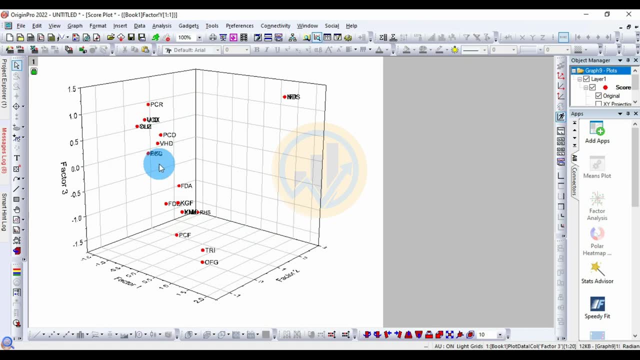 the next one plot for the square plot. open the plus icon. double click the square plot. this plot for the location for the pcr and pcd vhd also location the present in the factor three, the rh present in the center of the three factor. 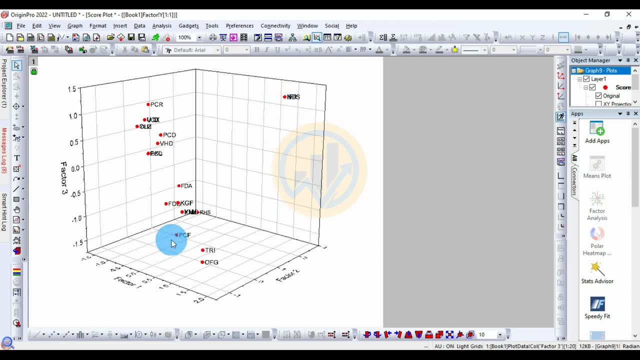 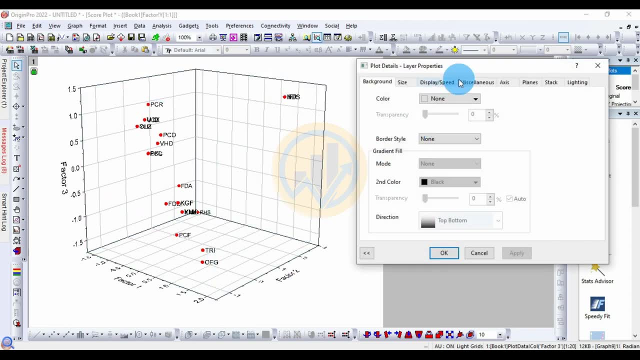 the nhp is a present in the single for the factor two, the pcf, tri and ofg also present in the factor one. double click for the center of the graph. open the new plot details. then click the panels the center of the grid line change. 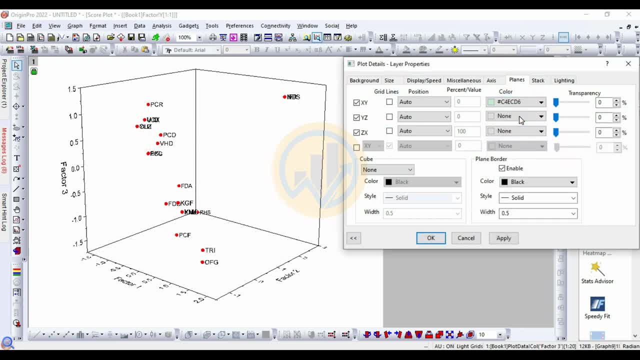 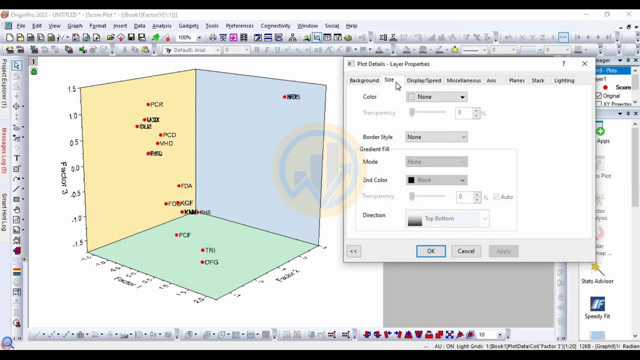 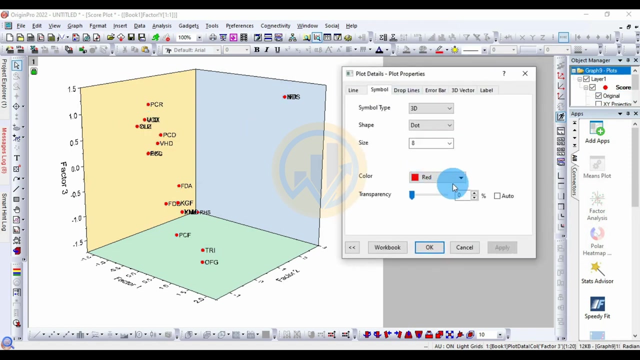 then apply change also the same method for the change color. then apply the difference color applied. then click double click for the center of the point. okay, double click the plot. it will open the change for the color dot, simple the color. 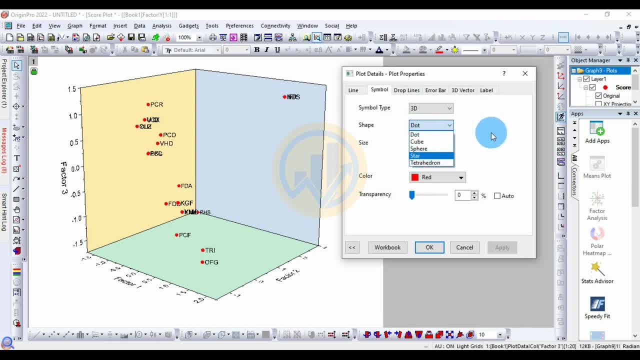 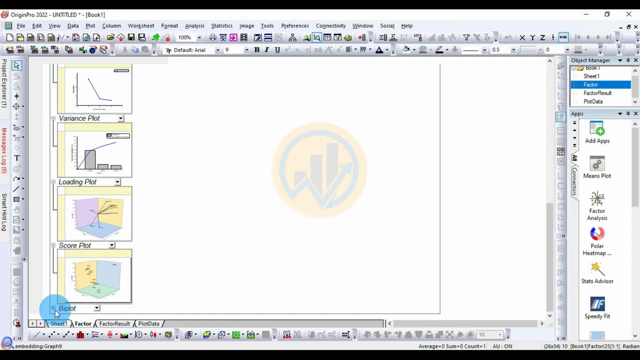 the next one for the change for the dot, cubic square and the star the change, then increase it for the size. okay, then increase the word size, then click the ok. the next one plot for the the biplot. the biplot presented in the double click for the center of the biplot. 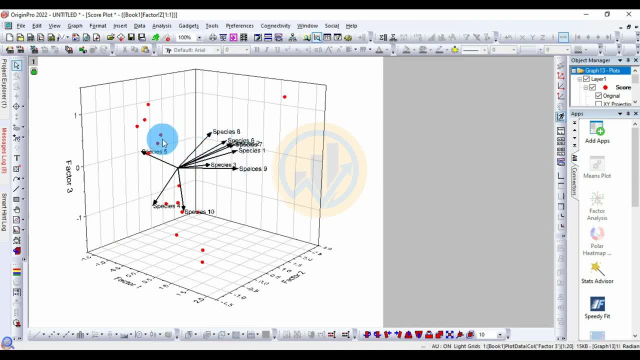 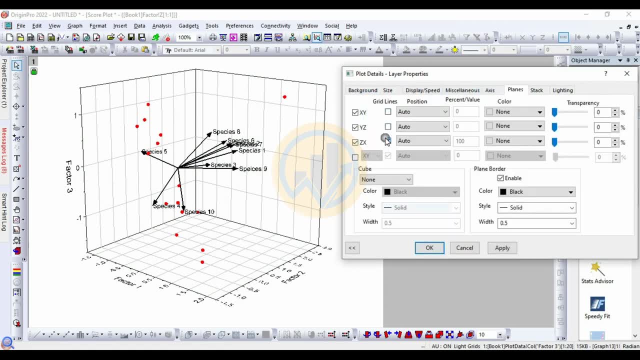 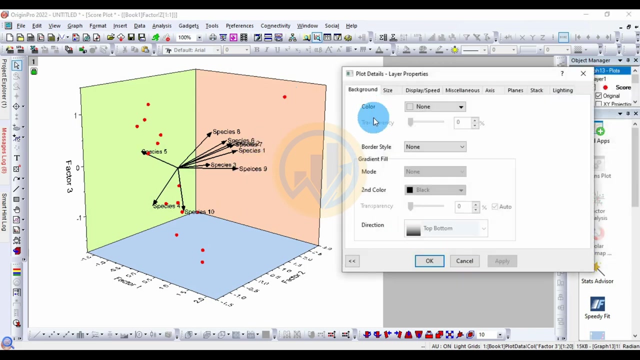 the biplot presented, the, the species data and the location data. the center of the double click for the chart, the panel, the. remove the grand lines. the change color then apply. this is a different color, same also the double click for the chart. 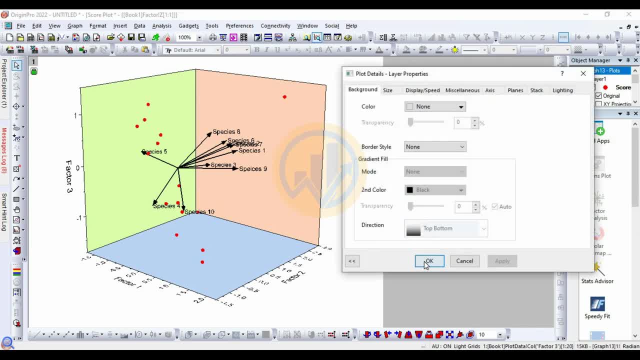 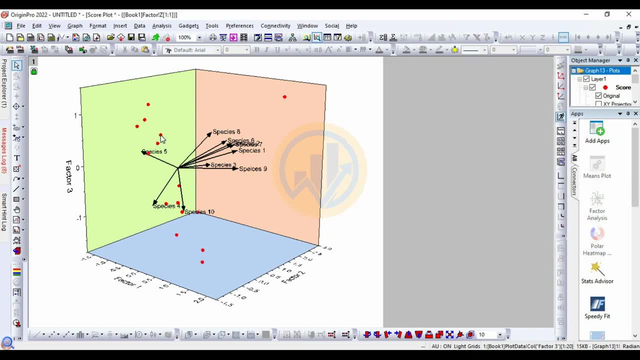 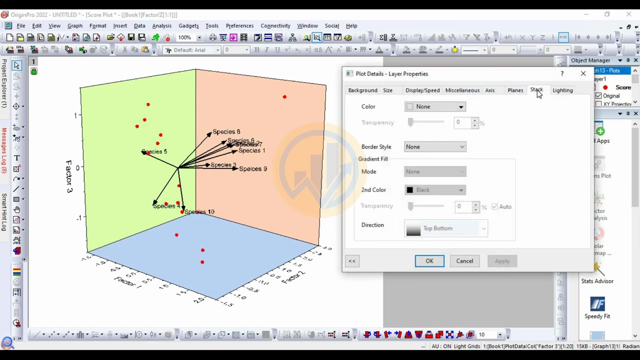 same also the double click for the, the dot. just change that. the palette will change later in the chart. okay, this one plot for the job over here. so for the top one, you did not get point color. you could not. you could universally. 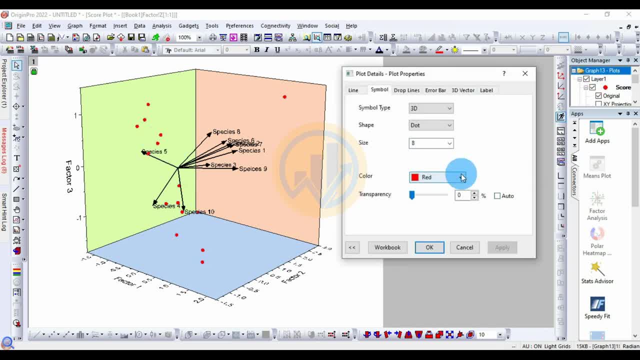 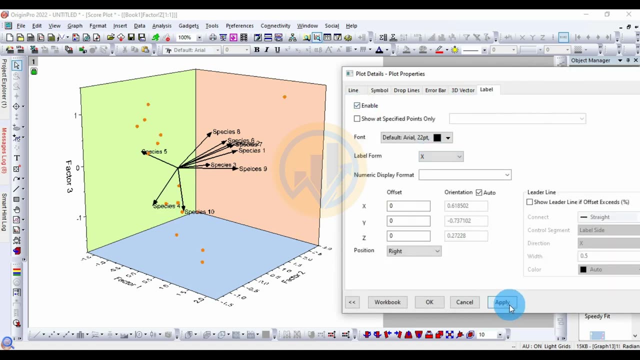 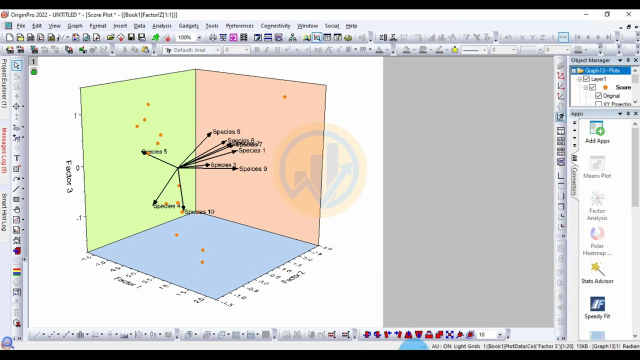 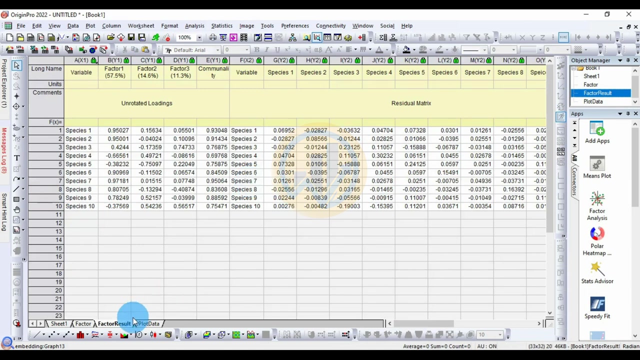 for example, let us say the formula, let us say that you take your concept color, dark or any other color, make it change the label, enable the label value for presented there. okay, then click the okay. the next one further, the factor resulting, the open, the fact of the center. the first one for the unrotated. 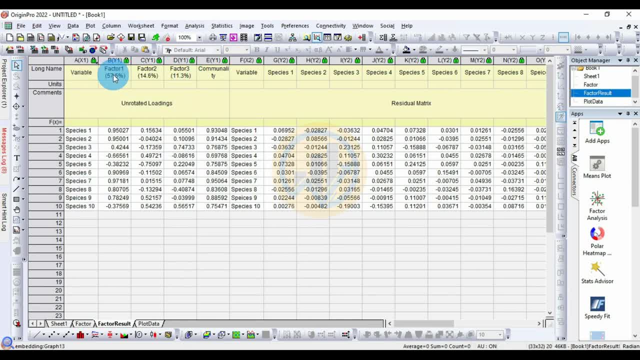 loading the very people on the factor 1, 2 & 3, the highest. also same for that, the loading blood. the loading blood is highest in the 57.5 and the second one of 14.6 that they're known for the 11.3 percentage. this is a species data: the power. 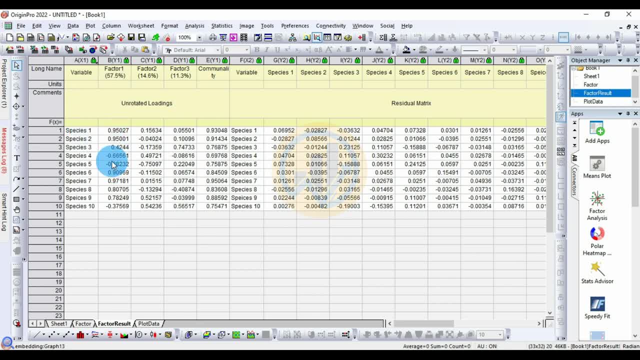 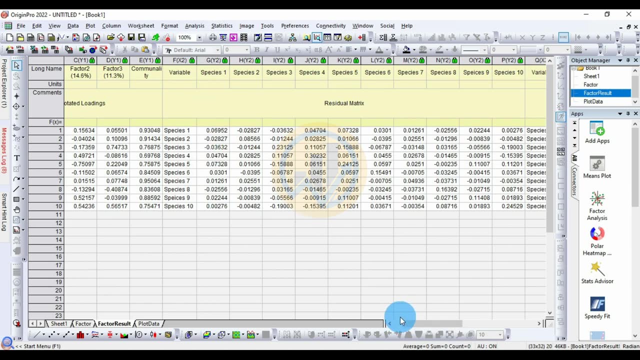 positively the factor 1, the result for the one species: 1, 2, 3 and this 6, 7, 8, 9, also the positive. the next one for the residual matrix value. this is resident where matrix value further species to species. then next one table. 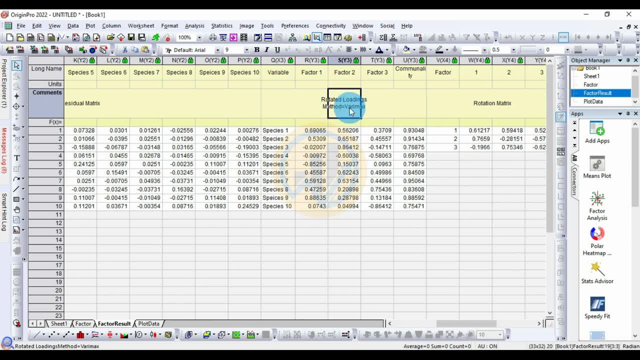 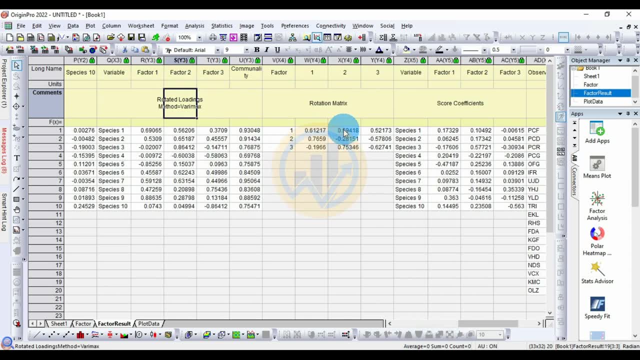 for the: the rotated loading semester matrix value: the factor 1, 2, 1, 2, 3 for the species. the next one for the table for the: the rotation matrix for the factor: factor 1 under to the 3, the highest to present in the rotation. 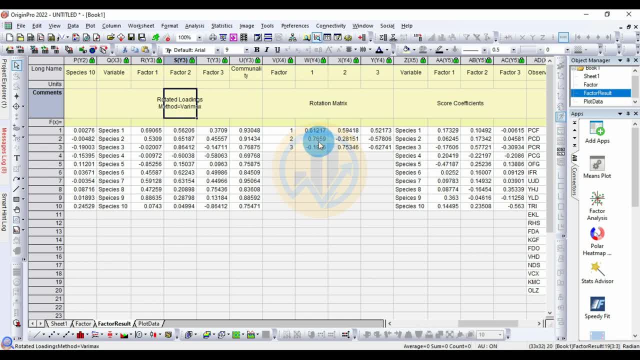 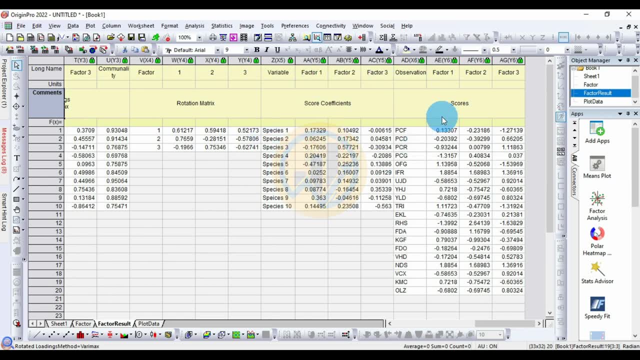 matrix in the value for the factor 2: 0 point seven, six point nine. then next one for the score of it against in the value the factor one, two, one, two, three for the, The species value, The next one. The philosophy table for that. 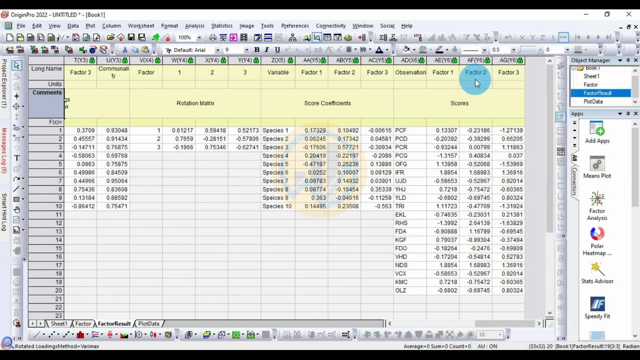 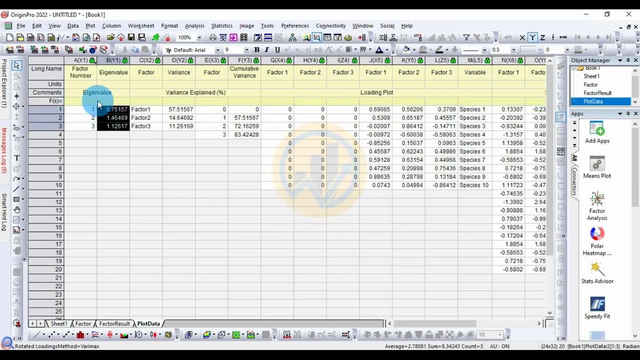 The score plot value The species and the factor 1,, 2, 3.. The score value, The next one. Data for the plot datas. The next one for the plot datas In the factor numbers And the eigenvalue. 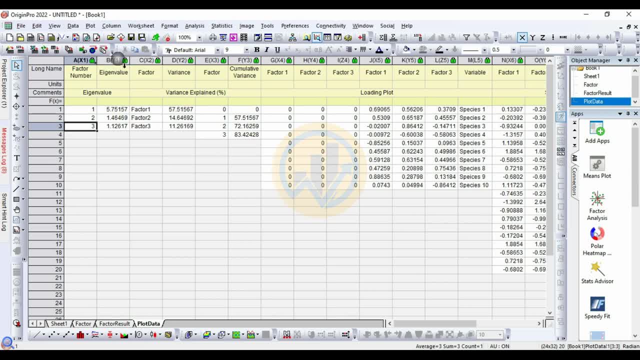 The factor 1, 2 and 3.. Then the next one for the eigenvalue, The next for the variation explained, for the factor 1.. And variation, the factor And the cumulative value. the next one for the loading plot value. this is a loading plot value, the factor. 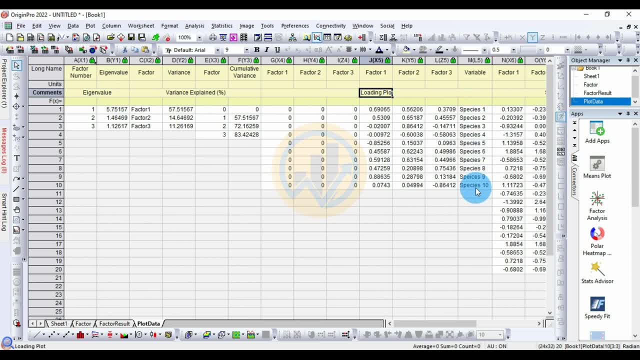 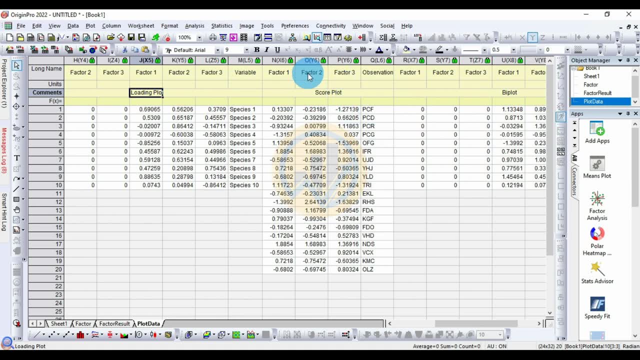 one, two, three. the factor one, two, three. the variable, the species. for the data and the loading plot value. the next one for the score value, the score plot for the species to the factor. the factor one, two and three. this is a factor value for the score plot. the last one for the by plot. this is by plot for the factor one. 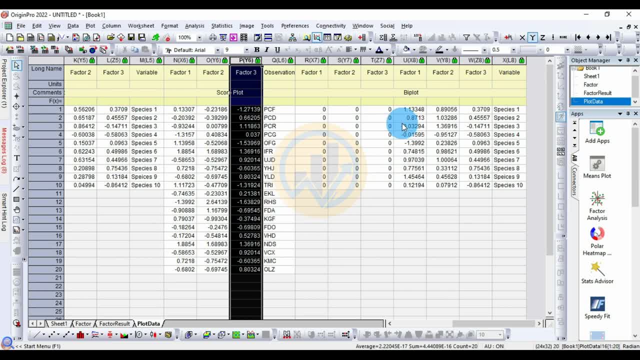 two and three for the species. this is a by plot value. thank you for watching this video.